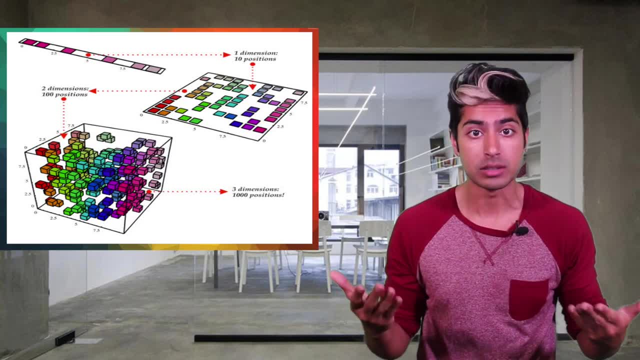 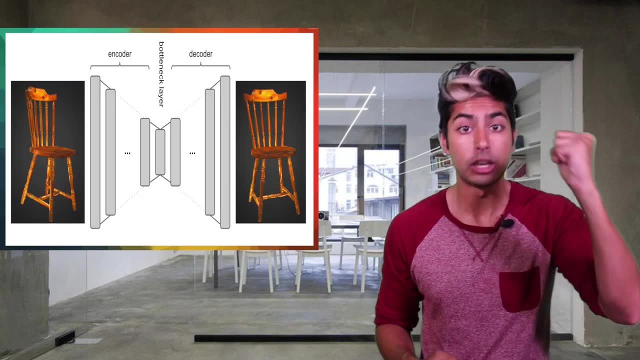 This reduces it to an m-dimensional space, so there are less dimensions. This process is called dimensionality reduction and it happens in every neural network. So we can think of the first layer as an image, The second layer of the network as the encoder, since it's compressing data. 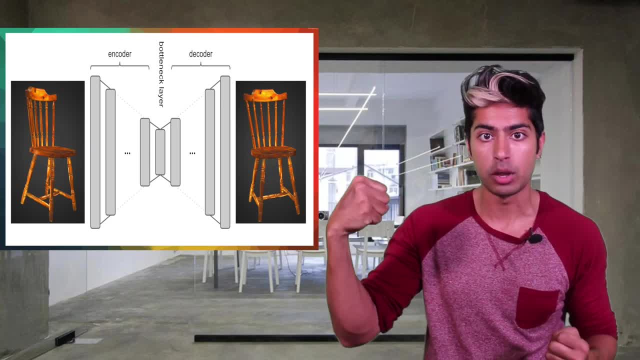 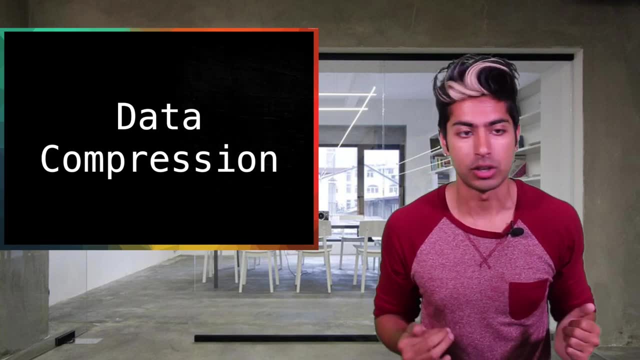 And the last part as a decoder, since it tries to reconstruct the original input from the smaller representations in the hidden layer. So when do we use autoencoders? All day, all day. Well, one use case is data compression, kind of like creating a zip file for some data set that you can later unzip. 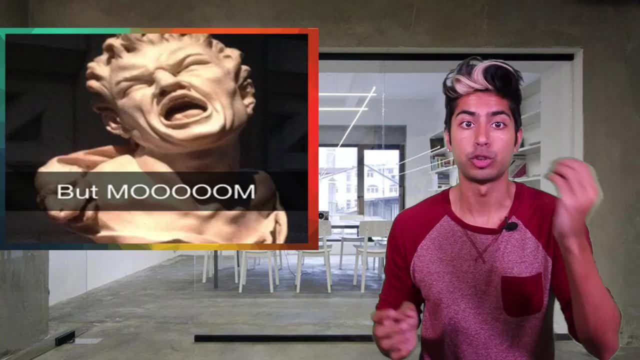 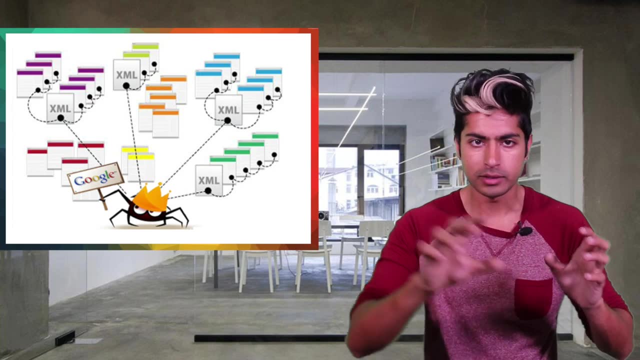 Another is image search, where you search Google using an image as your search query instead of text. It's very likely that Google is using autoencoders to help fuel this use case. Whenever one of Google's bots is crawling the web and finds an image, it'll compress it using an autoencoder. 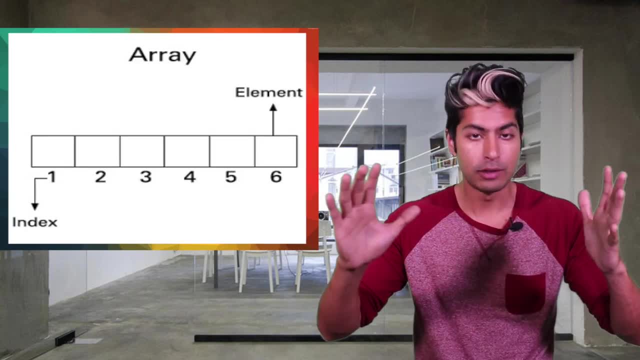 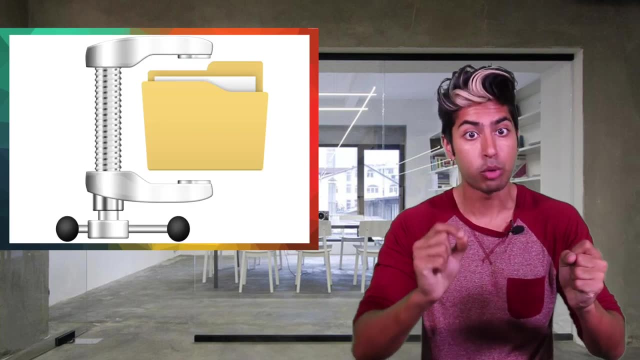 That would mean Google would have all of its indexed images compressed in the form of an easily searchable array. Whenever you search for a new image, it'll compress it and find all the points nearest to it in the compression space. since there is less noise, then rank them according to their similarity. 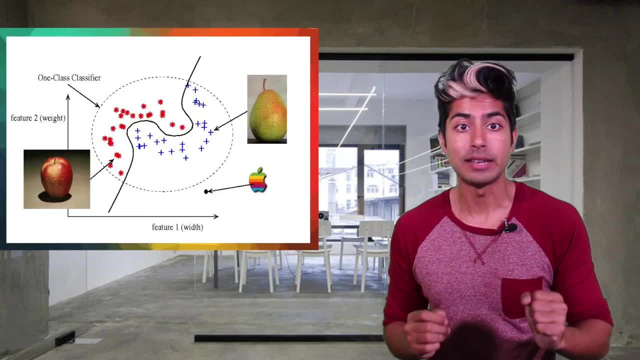 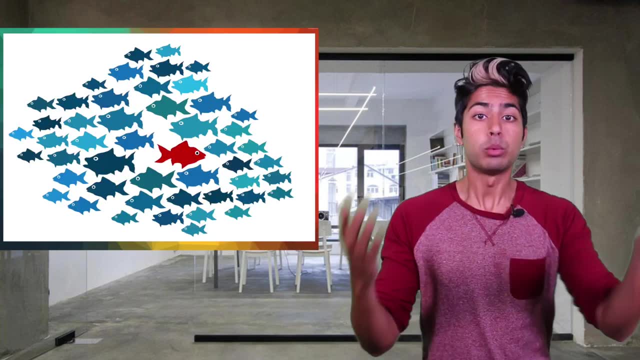 There's also the one class classification use case. That's when we only have a data set with a single class, which is called the target class. When we feed it to an autoencoder, it'll learn to detect objects of that class When it receives an object. 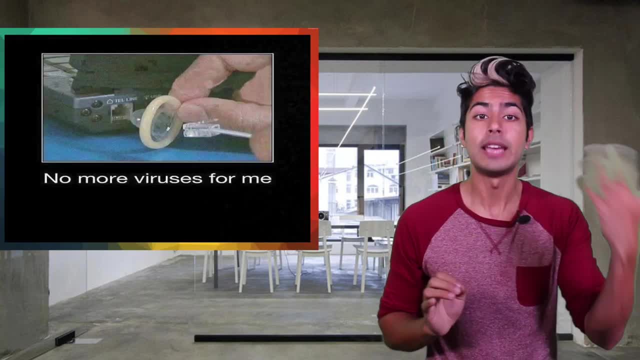 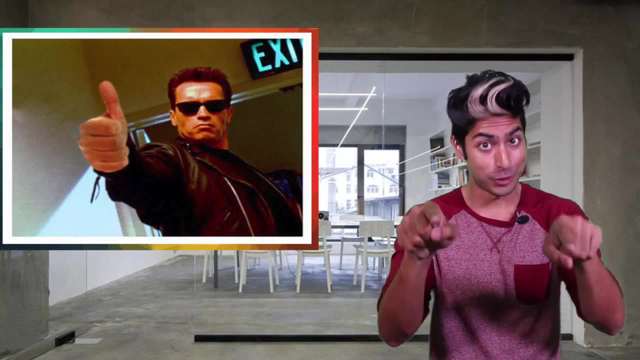 and doesn't fit that class category, it'll detect it as an anomaly, Whether it's a deadly virus or a fraud attempt, system downtime or someone who actually doesn't play Pokemon Go. That's right. autoencoders are for you. 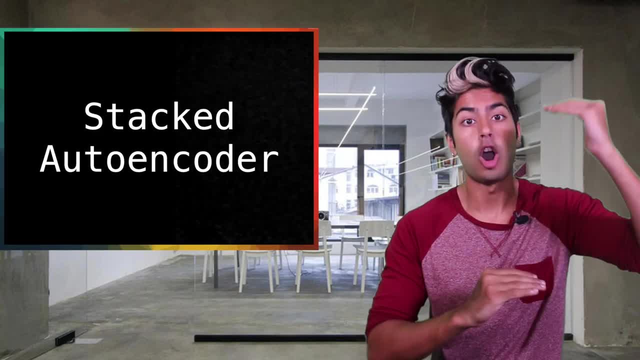 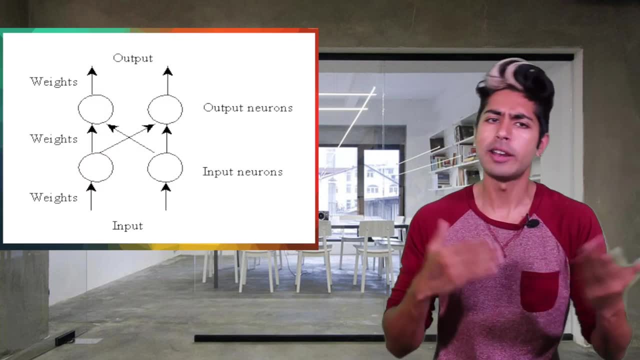 And if you want to train a deep network, you could use what's called a stacked autoencoder, That is, a set of autoencoders where the outputs of each layer are wired to the inputs of the successive layer. Once you train it on some data set, you can use those weights to initialize your deep net. 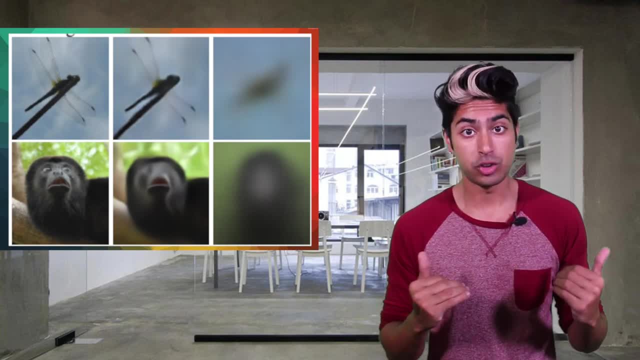 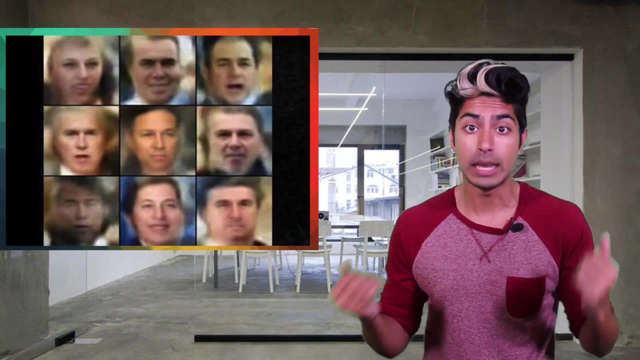 instead of randomly initialized weights. One of the more recent applications of autoencoders is generating novel, yet similar outputs to our inputs, Like faces that look really similar but are different than the input faces. For this we use a newer type of autoencoder called a variational autoencoder. 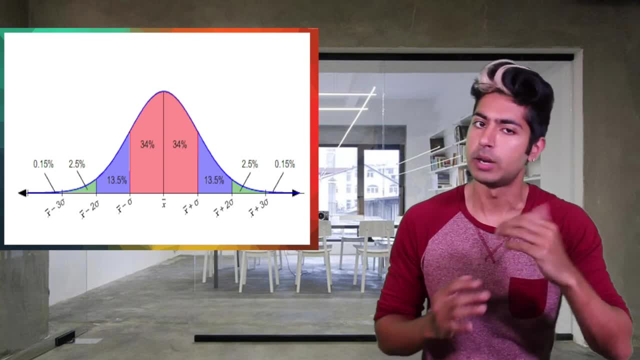 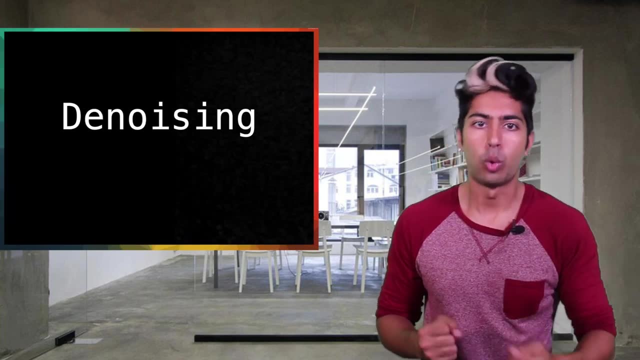 Which learns a distribution around data so it can generate similar but different outputs. There are lots of techniques that are used to prevent autoencoders from successfully reconstructing the input image, like denoising, where the input is partially corrupted on purpose. 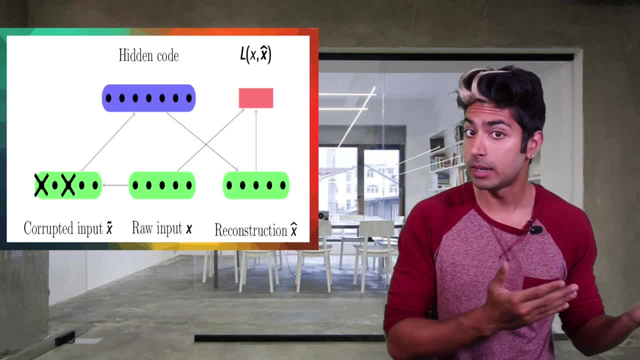 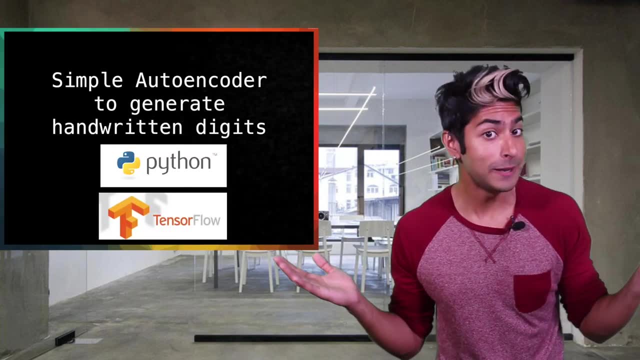 The idea is that if it can reconstruct an image despite it being corrupted, it'll be a more robust decoder. Let's build our own simple autoencoder to learn to detect handwriting digits using TensorFlow, shall we? First we'll import TensorFlow, the awesome machine learning library. 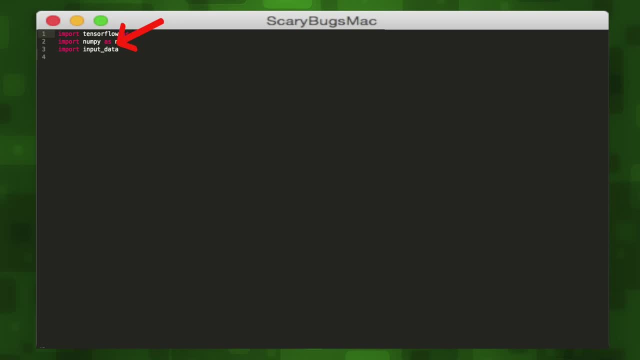 Then NumPy, the Pythonic scientific computing library. We'll also import our input data, which is the collection of handwritten character images. Then we'll define our autoencoder hyperparameters. We know that each character image is 28 by 28 pixels, so we'll set the width to 28.. 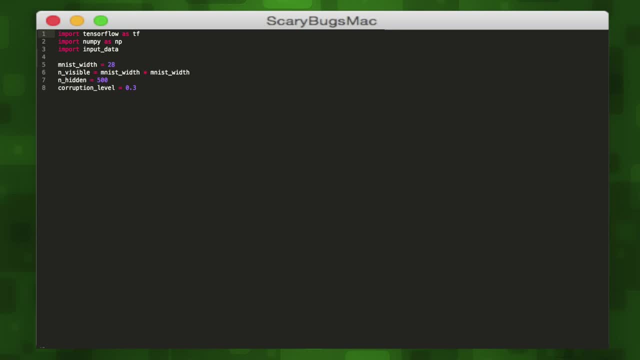 Then we'll initialize a variable that represents the number of input nodes. We also want to have 500 nodes in the hidden layer. I generally like to have 2 thirds the number of nodes in the hidden layer, My hidden layer as my input layer, as a starting point. 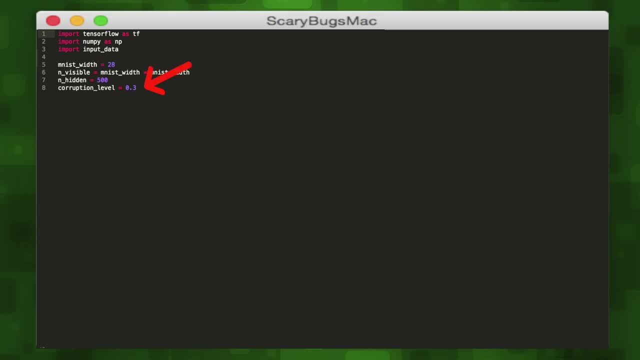 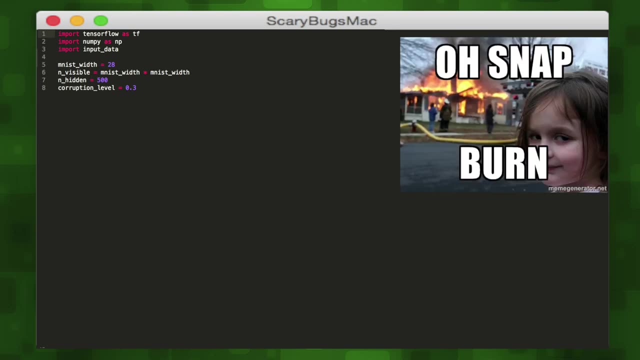 We'll want to purposely corrupt our input data later so that our decoder gets even more robust in its reconstruction over time. So let's set our corruption level to 0.3,, which isn't nearly as high as the US government's. Once we have these variables, we'll use them to help us build nodes. 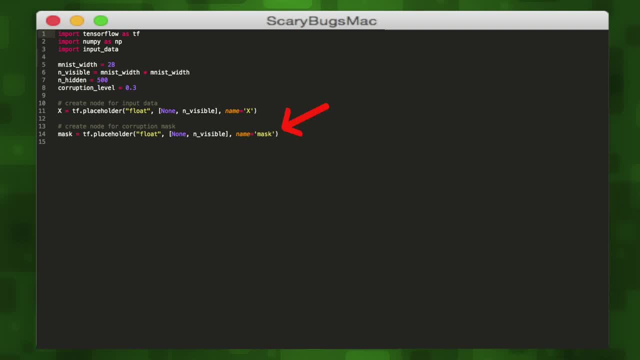 We'll start by creating a node for the input data. Then we'll create a node for the corruption mask, which will help us reconstruct the original image. We'll then want to create nodes for our hidden variables. After we initialize our weights, we'll initialize our hidden layer. 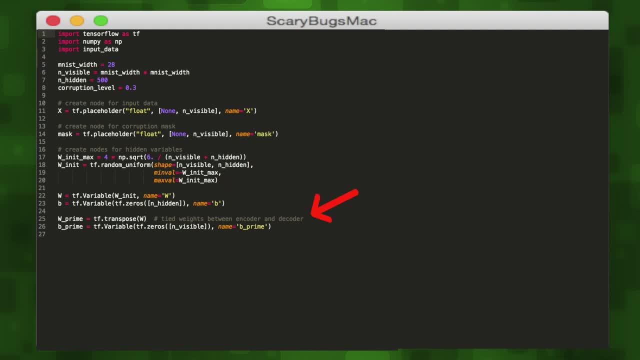 as well as the prime values for each that tie the weights between the encoder-decoder and result in an output value. After that, we define our model via a function that takes in our variable parameters. We'll make sure to get a corrupted version of our input data. 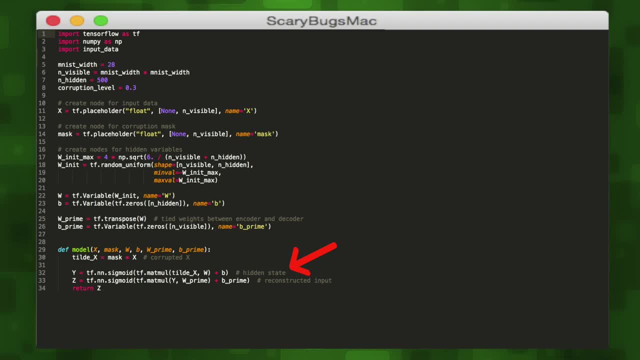 then create our neural net and compute the sigmoid function to create our hidden state. Then we'll create our reconstructed input and return that. So our model will accept an input and return a reconstructed version of it, despite the self-imposed data corruption. So we can utilize this function by building a model graph with it, which we'll call Z. 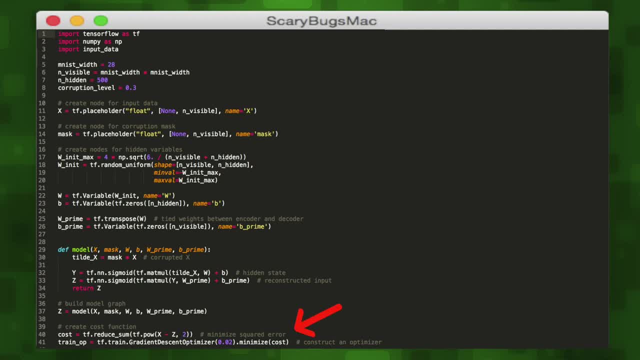 So, now that we have our model, we need to create a cost function, which is what we want to minimize over time. The more we minimize it, the more accurate our output results will be. Then we want to create a training algorithm, which we'll call trainOpt. 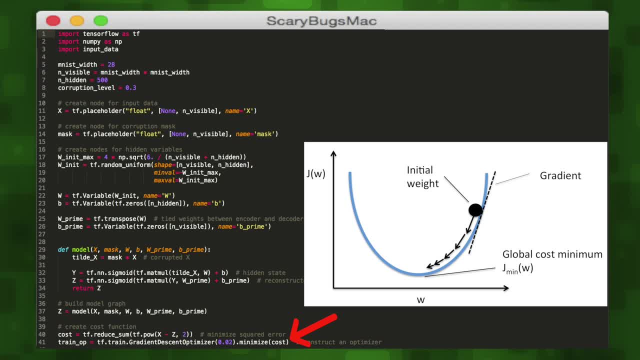 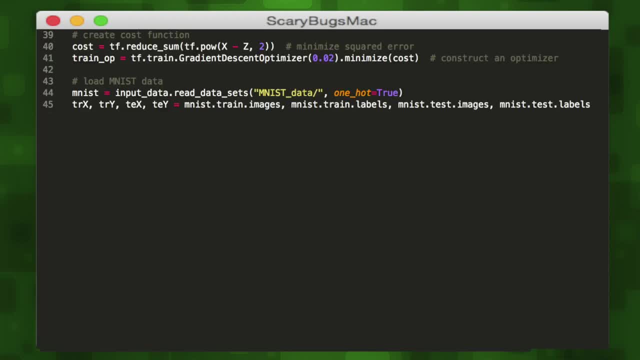 and use the classic gradient descent algorithm to help train our model, which takes the cost function as a parameter so it can continuously minimize when we train it. Before we start training our model, we need to load our data. so let's read from our local directory: